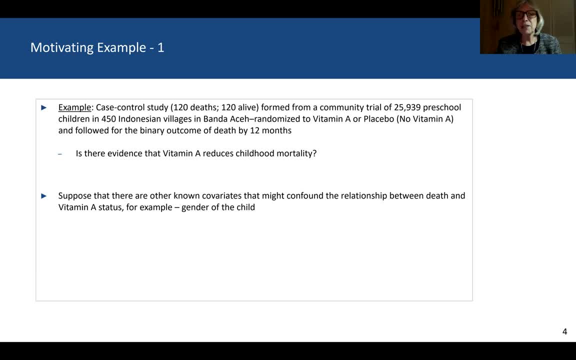 known covariates that might confound the relationship between death and vitamin A status, For example, gender of the child. So, just as a reminder, confounding occurs when there is an association between a covariate such as vitamin A status and mortality, as well as a relationship. 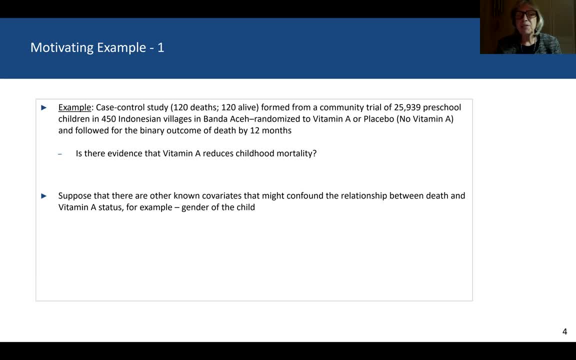 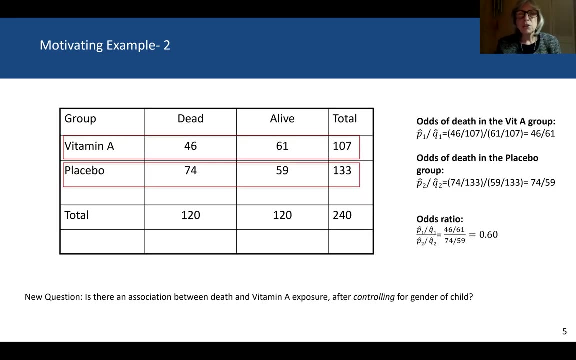 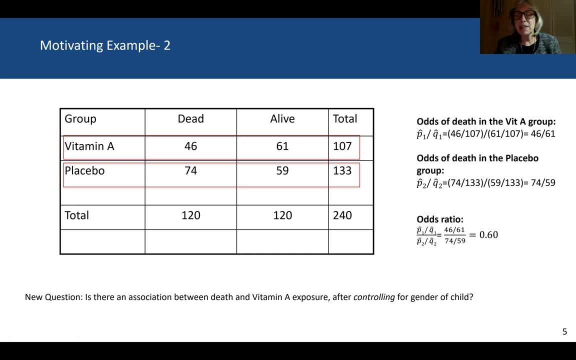 of the relationship between vitamin A status and case status, which is dead or alive. Here we can see that the odds ratio of death in the vitamin A group compared to the placebo group is 0.6.. This point estimate suggests a reduction of 40% in the odds of death. 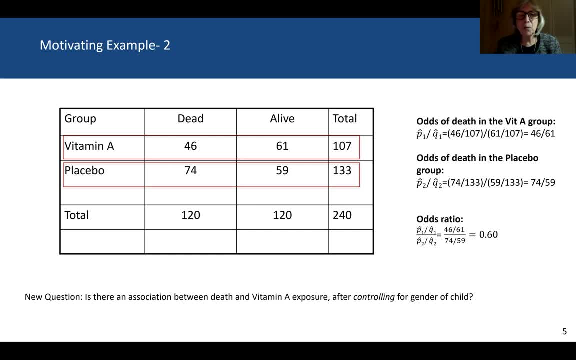 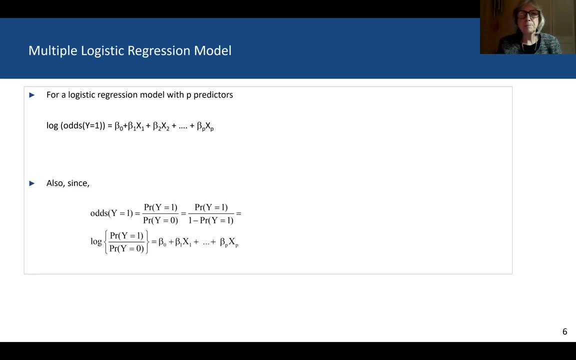 in the vitamin A group as compared to the placebo group. But this is now a new question: Is there an association between death and vitamin A exposure after controlling for the gender of the child? So for this we need a multiple logistic regression model that has 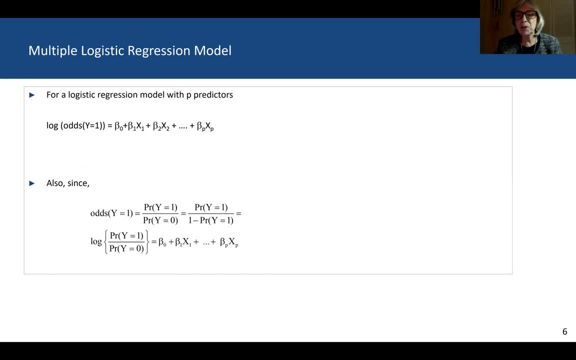 P predictors. In this case there will be just two predictors: vitamin A status and gender, And we would see that we would write the log odds model as a straight line relationship: beta 0 plus beta 1, X1, all the way through. beta P times XP And again P in this situation will be: 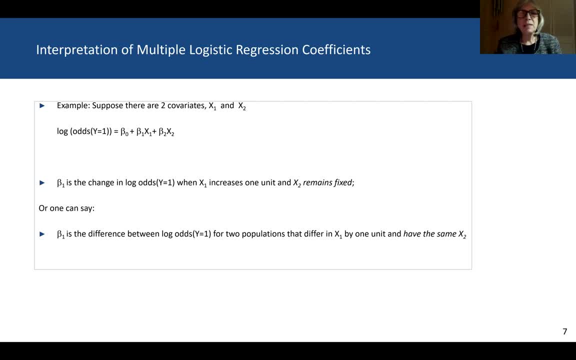 two covariates. So in the example of having two covariates- X1 and X2, we can determine or define the coefficients for those covariates. So let's start with looking at beta 1.. Beta 1 would be: 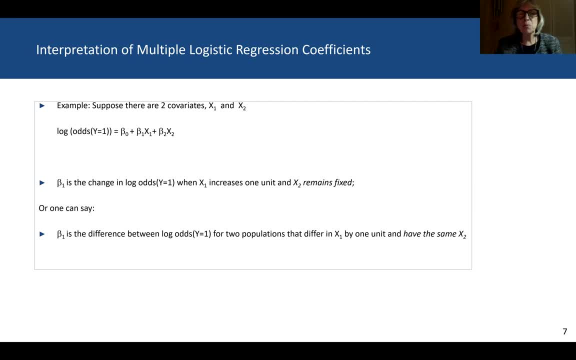 interpreted as beta 1.. Beta 1 would be interpreted as beta 2.. Beta 2 would be interpreted as beta 1.. The change in log odds when X1 increases by one unit and the value of X2 remains fixed, And when we say remains fixed, it's the same as saying X2 is adjusted for, controlled for. 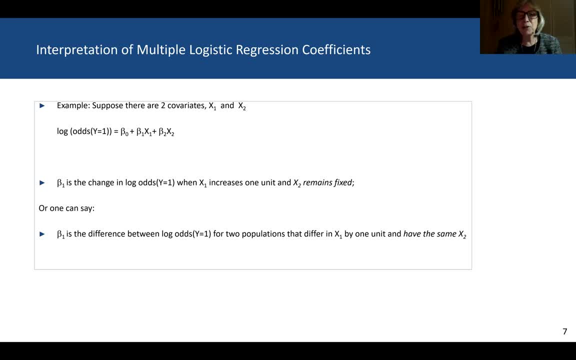 We're looking among individuals who have the same value of X2.. So all of these are synonyms for the value of X2 remaining fixed. So another way in which we can determine the value of X2 is by looking at the value of X2. 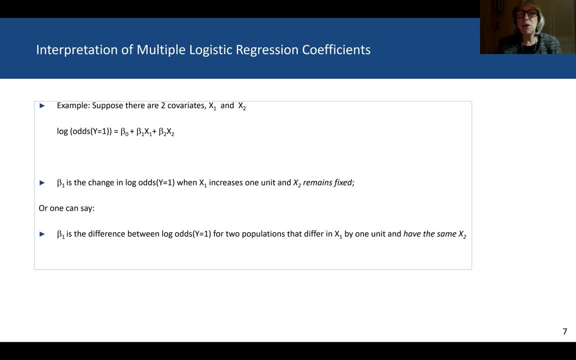 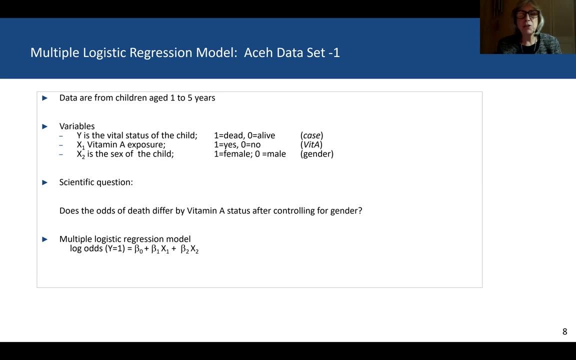 when X1 increases by one unit. And another way in which we can define beta 1 is that it's the difference between log odds for two populations that differ in X1 by one unit and have the same value of X2.. So let's look at the data setup for this multiple logistic regression using the data. 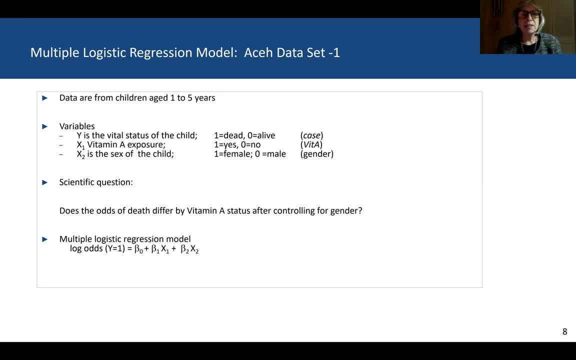 from Banda Ace. In this data set, the variables are that the variables are: Y- the outcome, which is the case or vital status of the child. 1 equals dead, 0 for alive. X1 is vitamin A exposure. 1 for yes, 0 for no. 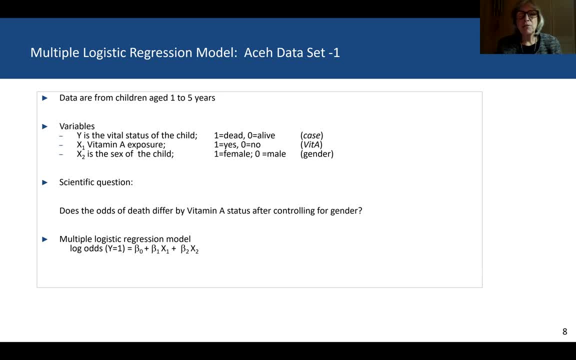 X2 is the sex of the child- 1 for female, 0 for male- which we will label as gender. And the scientific question is: does the odds of death differ by vitamin A status after controlling for gender? So this is a multiple logistic regression model. 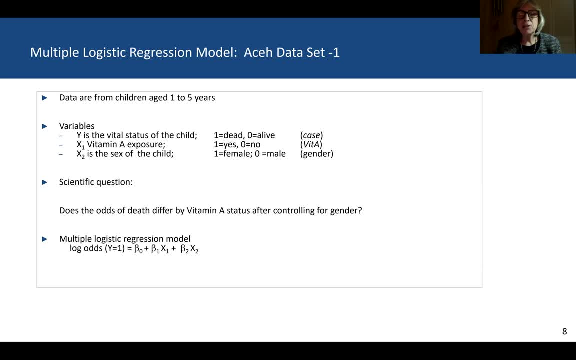 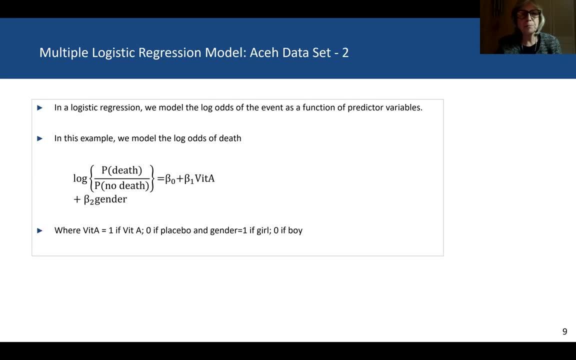 where we write the log odds of death is a straight line relationship: beta naught plus beta 1, X1 plus beta 2, X2.. So in this regression model we model the log odds of the event as a function of predictor variables And we keep in mind that vitamin A is coded as 1 if vitamin A, 0 if placebo. 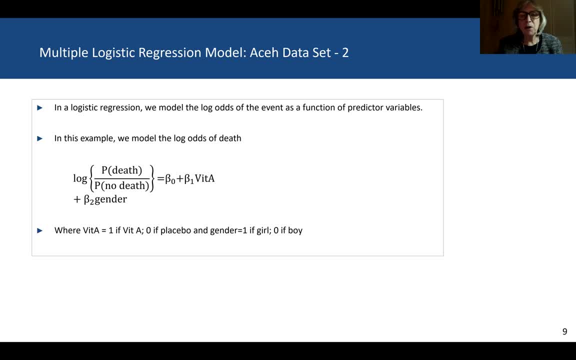 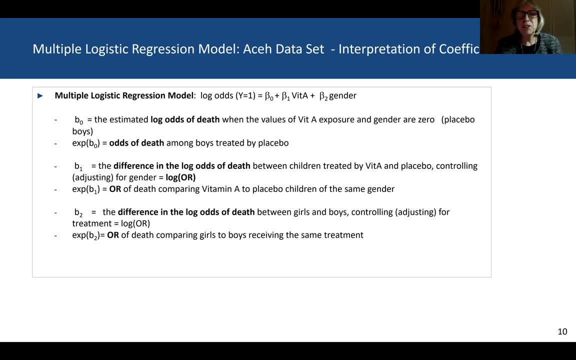 and gender is coded as 1 if a girl, 0 if a man, And we also model the log odds of death as a function of predictor variables. So the interpretation of our regression coefficients comes from inspecting the model that we see written. on this first line, The log odds of death equals beta naught plus beta 1 vitamin A. 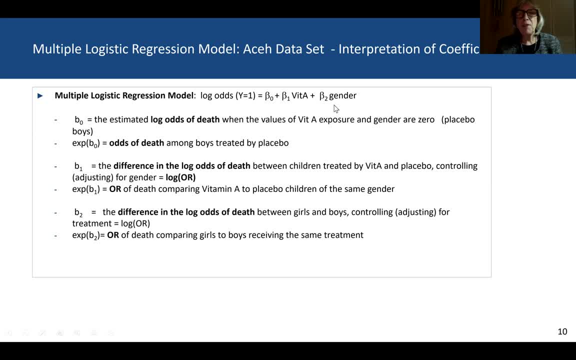 plus beta 2 times gender. So when vitamin A is equal to 0,, we're looking at the placebo group. When gender is equal to 0, we're looking at boys. So when those are both 0, beta naught, by definition, is the estimated well B naught. 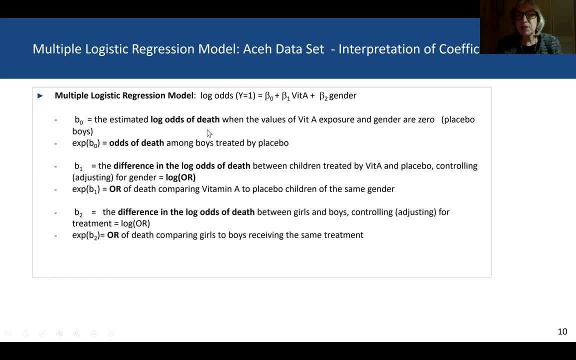 the estimate of beta naught is the estimated log odds of death when the values of vitamin A exposure and gender are both 0. So in other words, it's the estimated log odds of death among placebo-treated boys. If we exponentiate B naught, this will give us the odds. 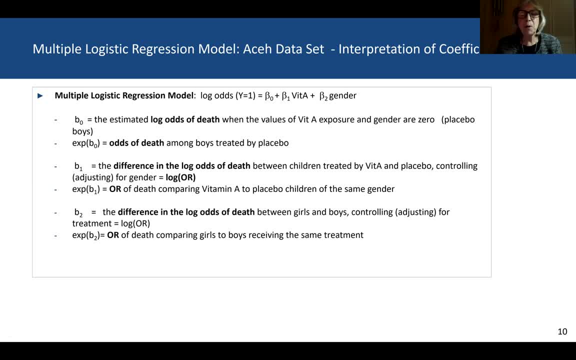 among boys treated by placebo. Beta 1 is the coefficient for vitamin A, So we know that B1, the estimate, is the estimated difference in the log odds of death between the children treated by vitamin A, where vitamin A is 1, and placebo. 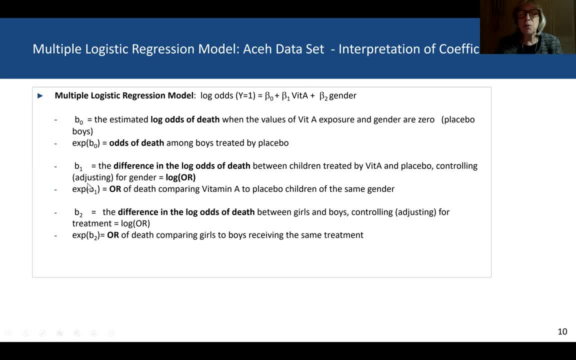 where vitamin A is 0, controlling for or adjusting for the other covariate of gender. So a difference in log odds of death is a log odds ratio. If we exponentiate B1, we obtain the odds ratio of death comparing vitamin A to placebo children. 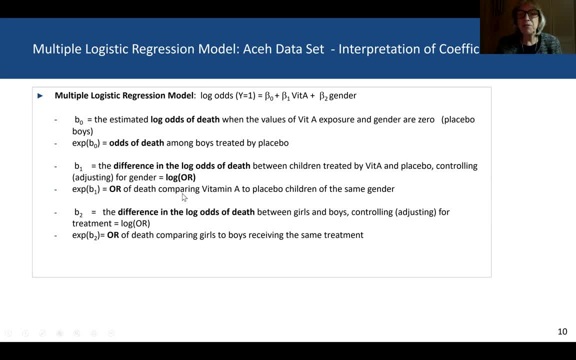 of the same gender, meaning we're fixing the value of gender, we're adjusting for it, we're controlling for it. B2,, the estimated coefficient- the estimate of the coefficient beta 2, is the estimated coefficient for B1. So if we exponentiate B1, we obtain the odds ratio of death. 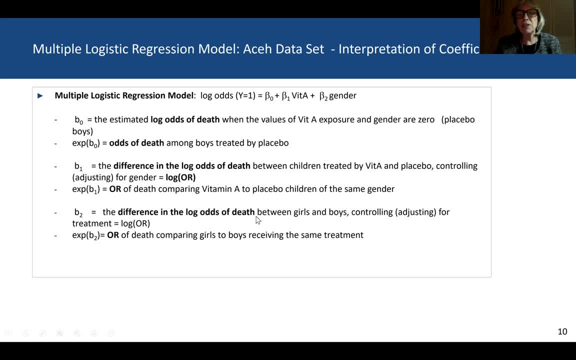 the coefficient for gender is the difference in the log odds of death between the group of gender coded 1,, which is girls, and the group coded 0,, which is boys. controlling for or adjusting for treatment, In other words, vitamin A status. B2 is a log odds ratio And if we exponentiate B2,. 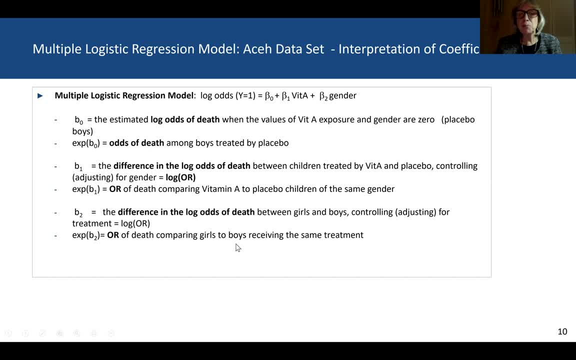 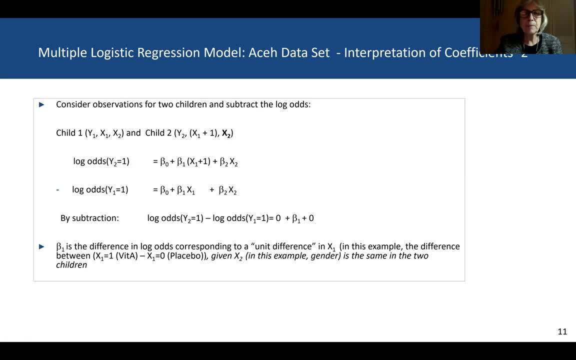 it is the odds ratio of death comparing girls to boys who have received the same treatment, meaning treatment is fixed. So just to make sure that we believe that this interpretation of beta 1 is a log odds ratio, we can consider two children: child 1,, who has the outcome, Y1,, who has a covariate of the value. 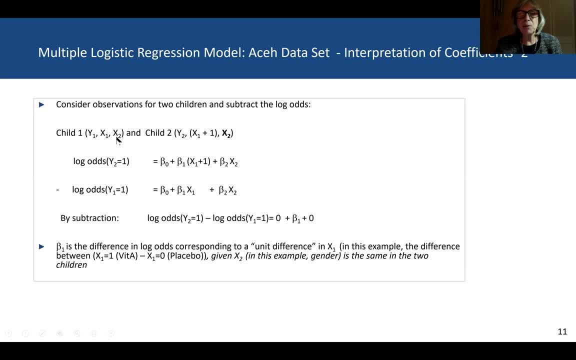 X1, and the second covariate has the value X2.. So child 2 has the outcome Y2, its value of X1 is increased by one and it has the same value of the covariate X2.. So we can write for child 2, the log odds of death. 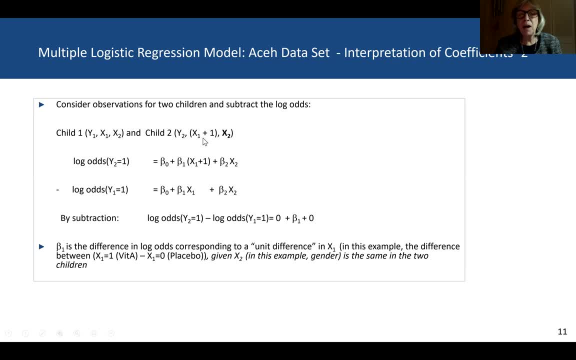 equals beta 0, plus beta 1, times X1, plus 1, plus beta 2, times X2.. Whereas for child 1, we would write: the log odds of death equals beta 0, plus beta 1 x1 plus beta 2 x2.. If we subtract these two log odds, the beta nots cancel out. 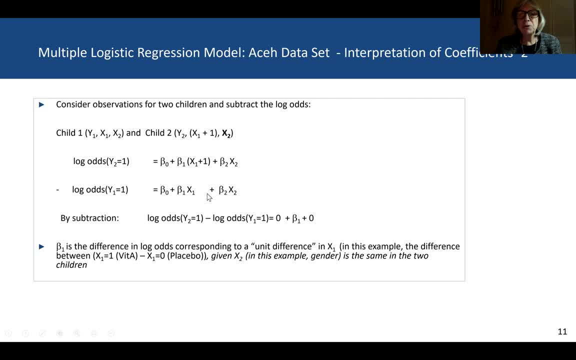 beta 1 times x1 cancels out, and beta 2 times x2 cancels out. So we're left with a difference in the log odds of death in child 2 minus the log odds of death in child 1, which reduces to beta 1.. 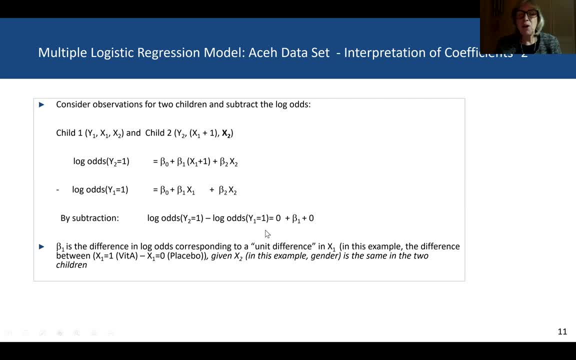 So a difference in log odds is the same as the log of their ratio. But we'll just be explicit here that beta 1 is the difference in the log odds. that corresponds to a unit difference in x1.. In this example, the difference is between: x1 equals 1, which is vitamin A. 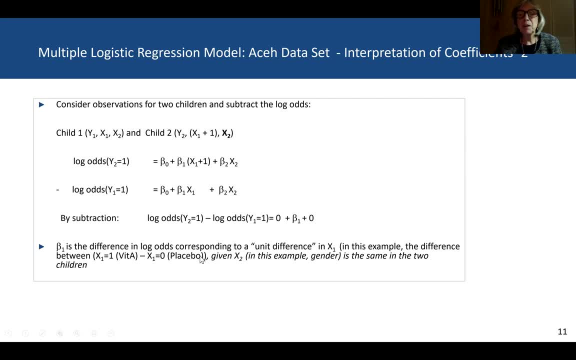 and x1 equals 0,, which is placebo. So it's the difference in the log odds between those treated by vitamin A and placebo, given that gender is the same. So adjusting for or controlling for gender, And if we exponentiate beta 1, we get the odds ratio of death in vitamin. 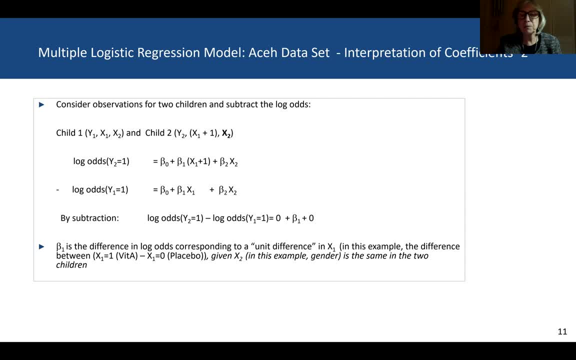 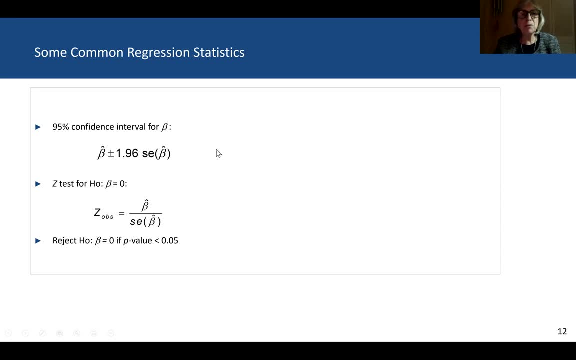 A versus placebo. controlling for gender. We use the same regression statistics we've used for different models in which we can see that the odds ratio of death in vitamin A versus placebo is the same. We can set up a 95% confidence interval for the true beta by taking the estimated beta. 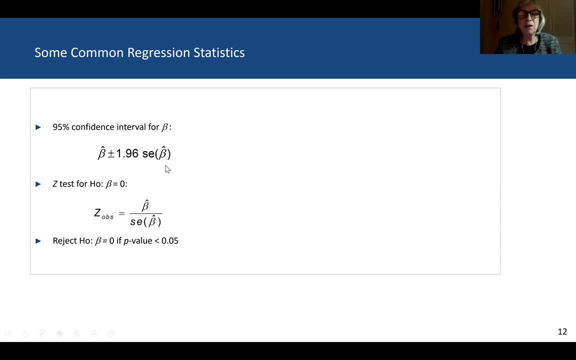 plus or minus 1.96 times the standard error of the estimate. We can set up a z-test to test that beta equals 0, and that observed z-statistic takes the estimated beta minus 0 divided by the standard error. We would reject the null hypothesis if our p-value for this observed z-statistic is: 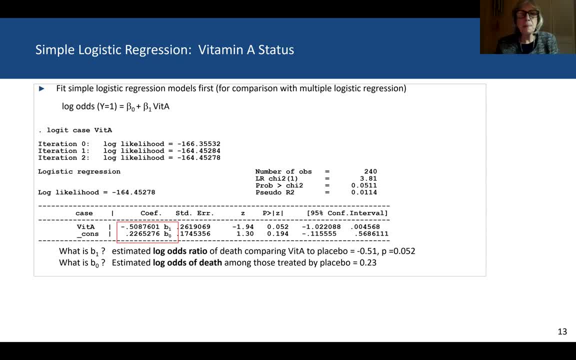 less than 0. So we can set up a 95% confidence interval for the true beta by taking the estimated beta less than 0.05.. So let's first look at the simple logistic regression models for each of the independent covariates. First we'll look at vitamin A status. We'll fit the model that the 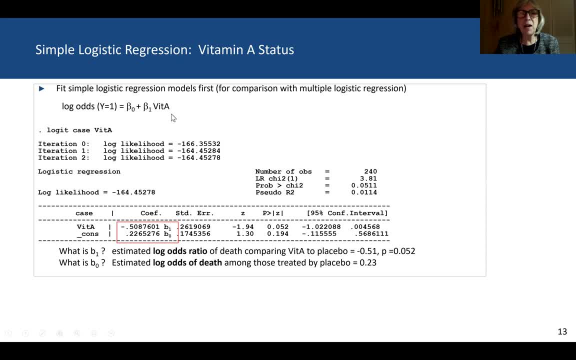 log odds of death equals beta naught plus beta 1 times vitamin A. We see the coefficients that are estimated here, B1 and B naught, And we would answer the question of what is B1 by saying it's the estimated log odds ratio of death comparing vitamin A to placebo. 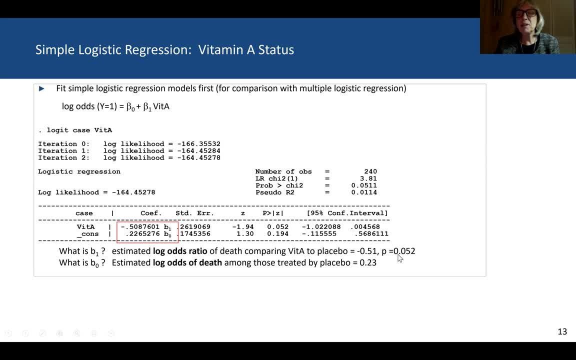 And we see that value is negative 0.51.. The p-value is not statistically significant. It equals 0.052.. The way we would get the odds ratio would be by exponentiating negative 5.07 to give us the odds ratio of death. comparing vitamin A to placebo. 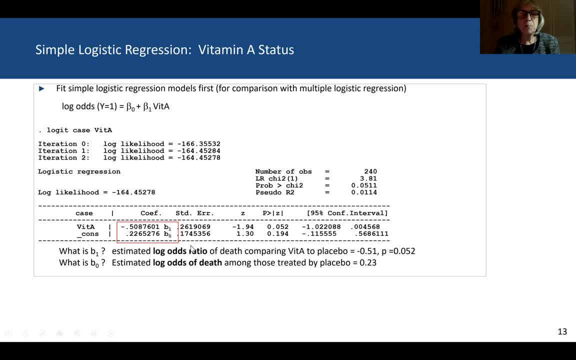 And, for the purposes of completeness, we can answer the question: what is B naught? It would be the estimated log odds of death among those treated by placebo. In other words, vitamin A would equal 0. This cancels out And B naught by itself is the log odds of death among those. 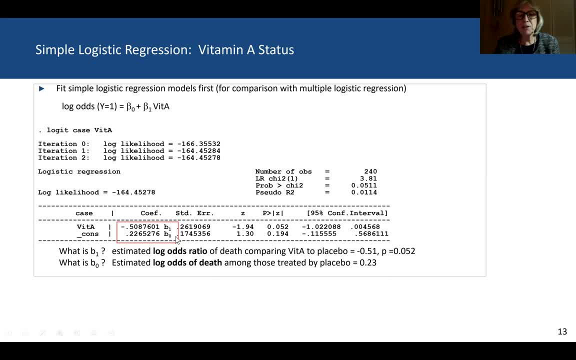 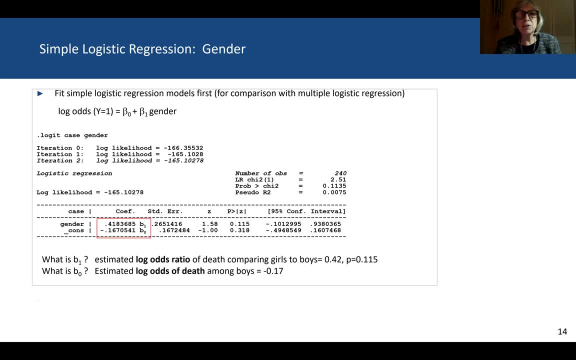 treated by placebo, And that value here is 0.23.. Let's also look at the simple logistic regression by gender. So here we would fit the model log. odds of death equals beta naught plus beta 1 times gender. We look down to see the estimated. 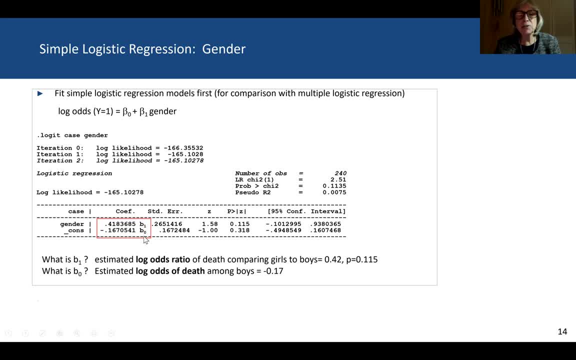 coefficient B1 for gender and the estimated intercept B naught. And to answer the question, what is B1?? It would be the difference in the log odds of death Between the group coded 1,, which is girls, and the group coded 0,, which is boys. In other words, 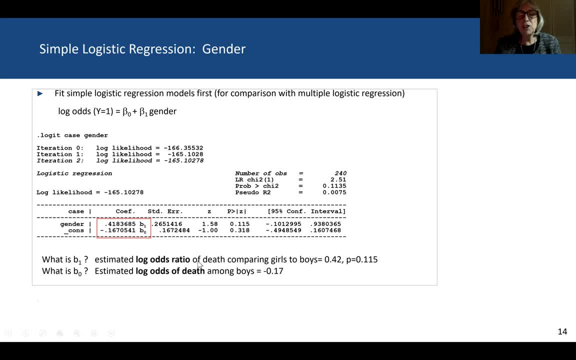 that difference in log odds is a log odds ratio of death. comparing girls to boys, We see that that's estimated by 0.42.. And the p-value is 0.115.. So there's no statistically significant difference in the log odds of death between girls and boys. 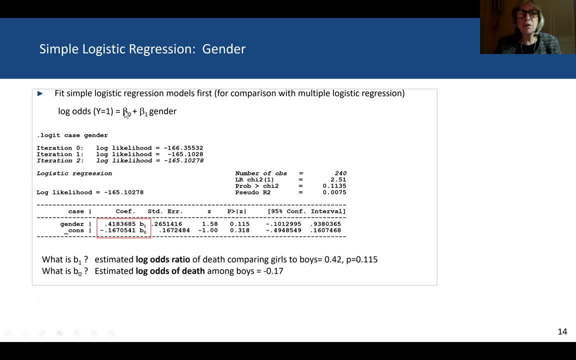 And again for completeness, when gender is equal to 0, beta 1 times 0 cancels out. Beta naught is the log odds of death among boys And we would say that B naught is the estimated log odds of death. 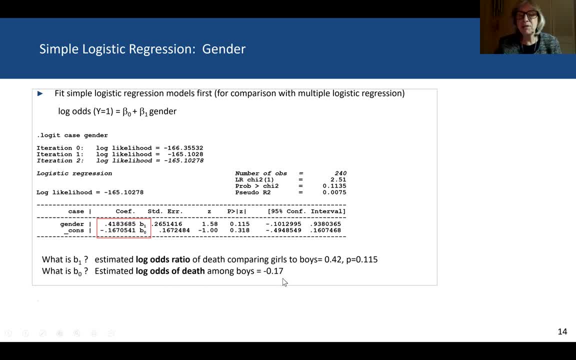 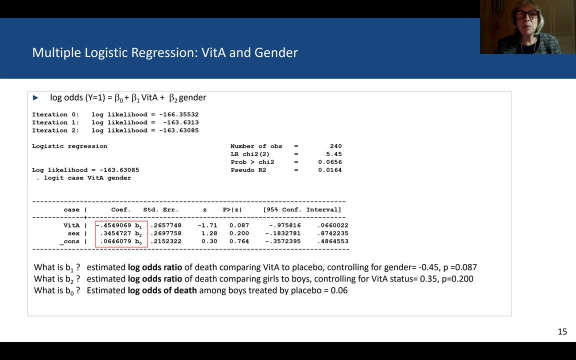 among boys And that value is negative 0.17.. Now what happens if we fit a multiple logistic regression model with both vitamin A and gender? We see the model is now written. the log odds of death equals beta naught plus beta 1 vitamin A. 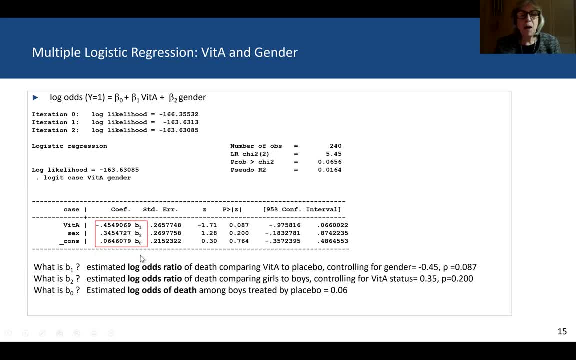 plus beta 2 times gender. We see in the box the estimated coefficients B1,, B2, and the estimated intercept B naught. And our interpretation of these coefficients now is that B1 is the estimated log odds ratio of death comparing vitamin A to placebo controlling. 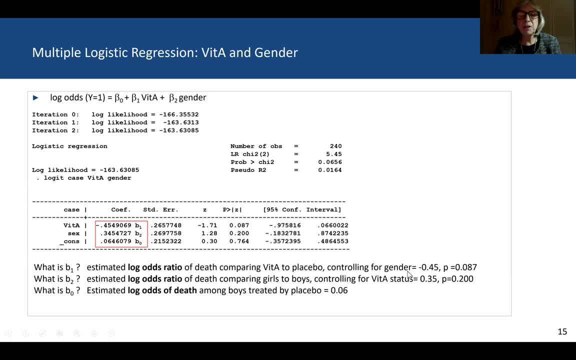 for gender Meaning among children of the same gender. That coefficient has a p-value of 0.087.. And we would conclude: there's no statistically significant difference in the log odds of death between children treated by vitamin A versus placebo after accounting for or adjusting for gender.